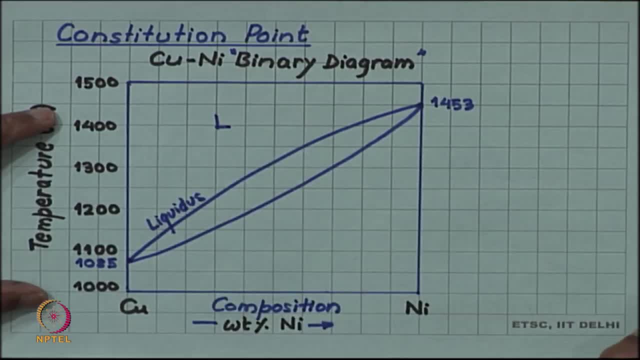 And above that we have a liquid phase which is in equilibrium. the lower boundary is a solidus boundary and below this a solid solution phase is stable. and we have established this convention- and this is quite common- that the solid phases we will represent by Greek letters. 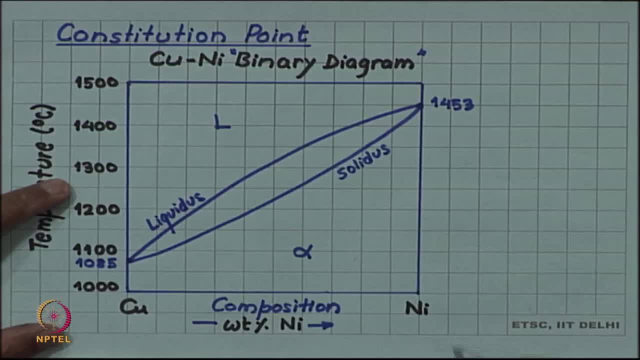 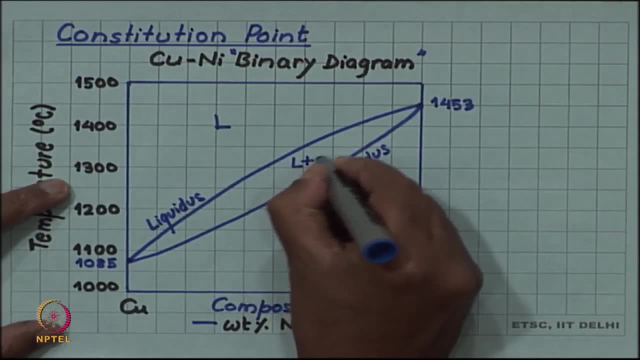 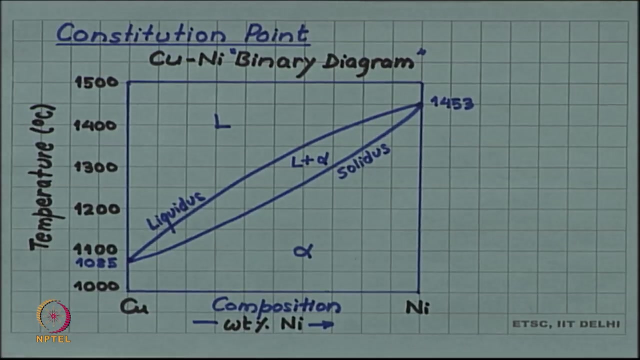 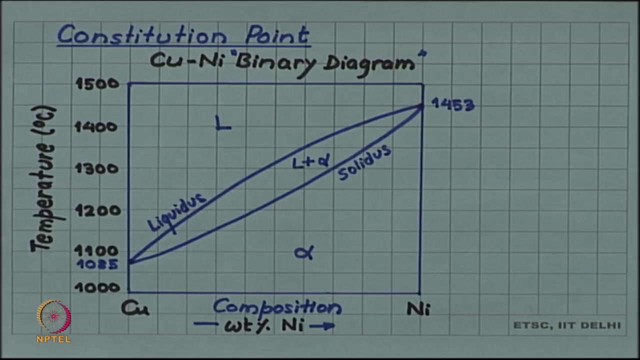 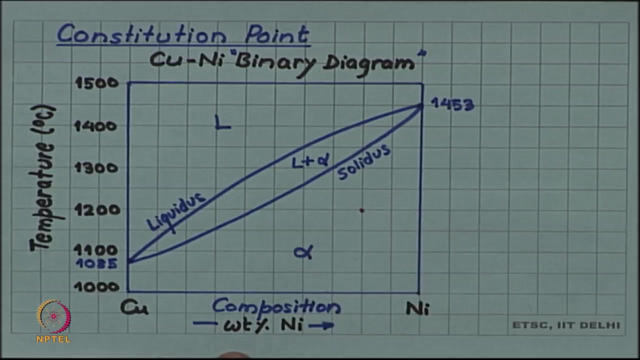 So I have written alpha for this particular solid phase And in between the two boundaries we have a two phase region, liquid plus alpha. So we have seen this in the last discussion. Now this phase diagram is a diagram in the composition temperature space. So any point in the diagram if I mark, any point, if I put my pen at this, 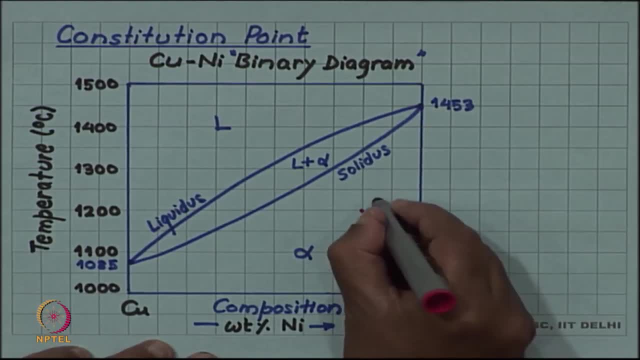 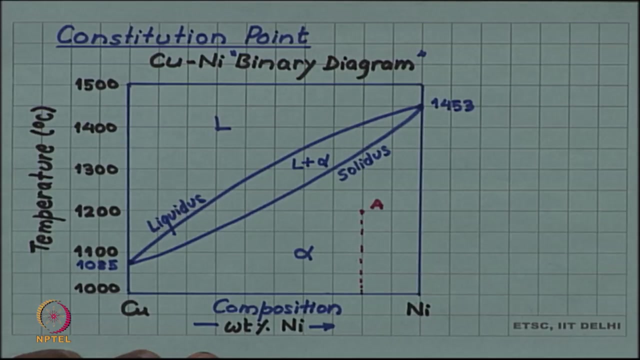 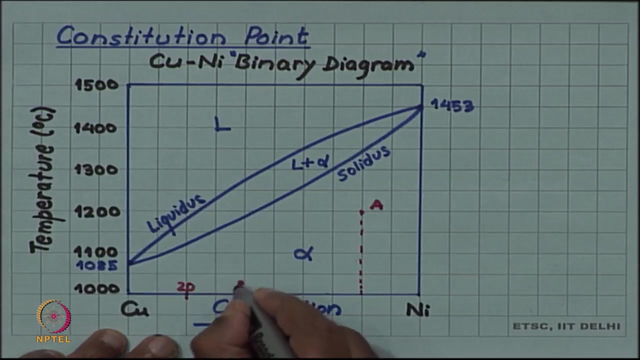 point. Let me call this point A. So this point represents, since it is a point in temperature composition space, it is x coordinate. the x coordinate of this point is a composition. In this particular case, you can see that if I try to find out its composition, it is easy. 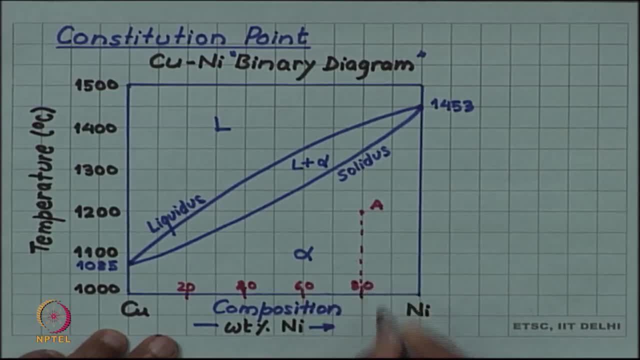 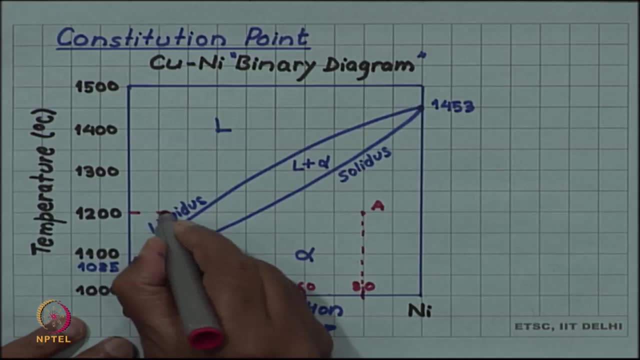 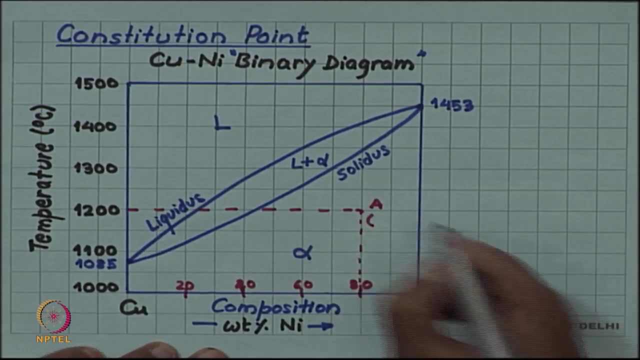 So it is 80.. 80.. 80 weight percent. nickel is what is its x coordinate and its y coordinate is a temperature, And in this case again, the temperature is 1200 degree Celsius. So this particular point represents an alloy of 80 weight percent. nickel: 80 weight percent. 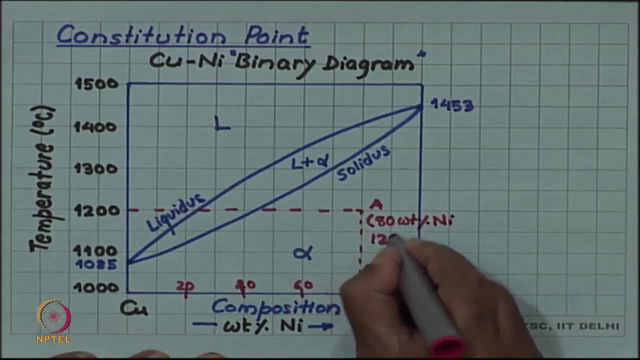 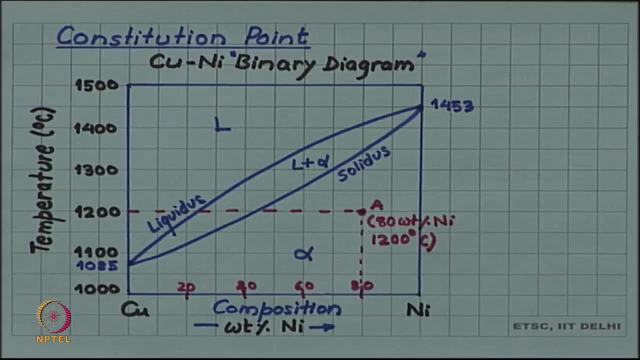 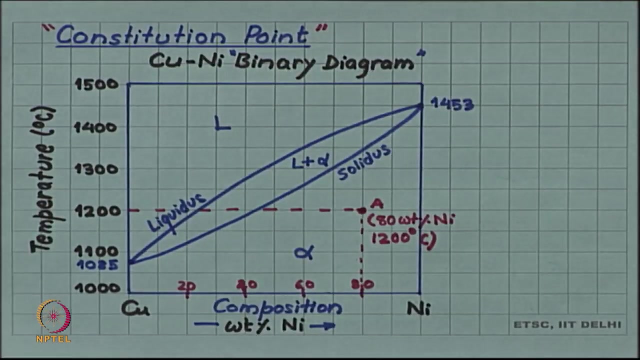 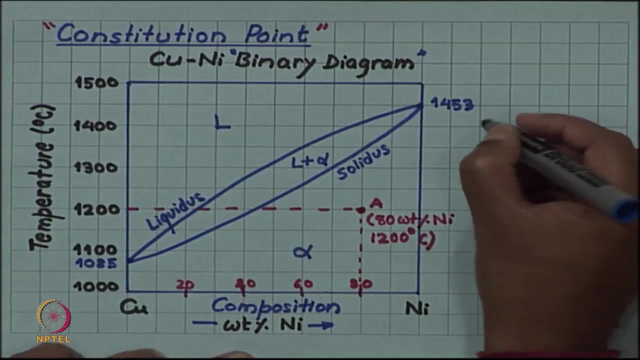 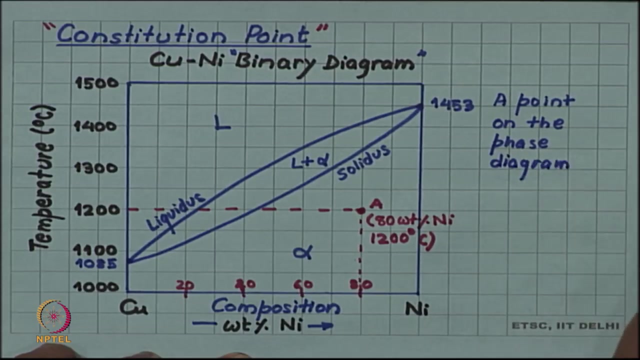 nickel, And this is the equilibrium at 1200 degree Celsius. So such points, which are the points of our interest, we will call constitution point. So any point in the phase diagram can be a constitution point. So a point, a point on the phase diagram, let us say a point x, t, where x is the composition. 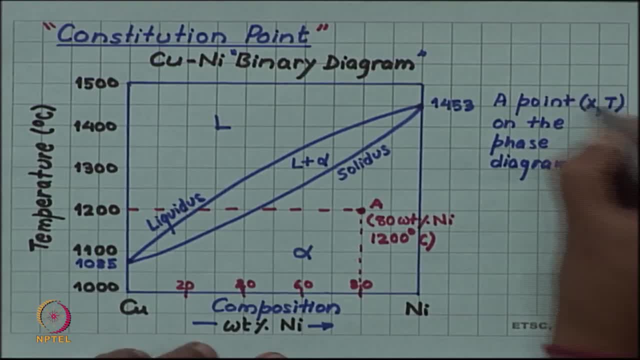 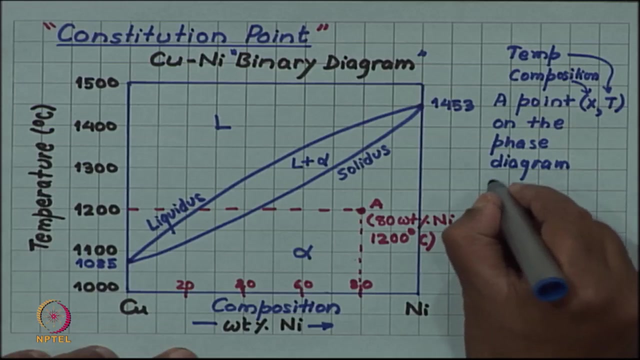 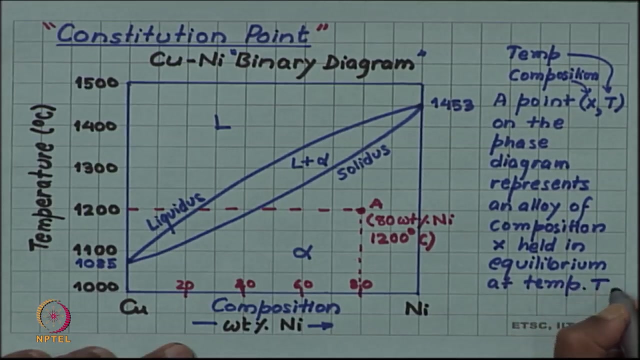 And T is the temperature. x is the composition and T is the temperature. So any point x, t in the phase diagram represents77 sevent and watts. Okay, Hey, an alloy of composition x held in equilibrium at temperature T, and that is the point which I am for the moment naming as constitution. 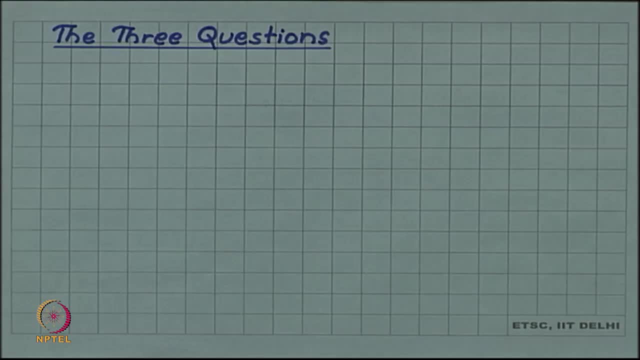 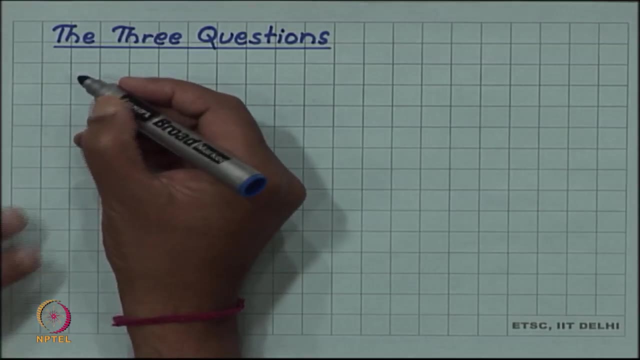 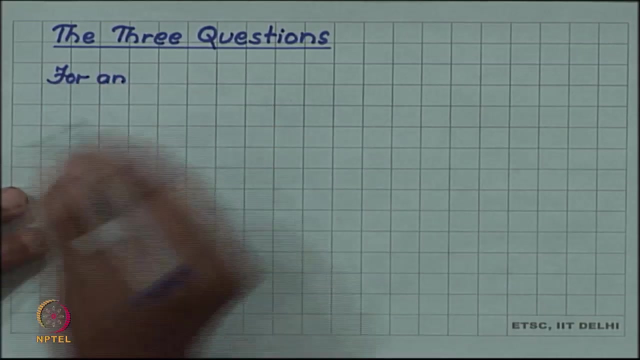 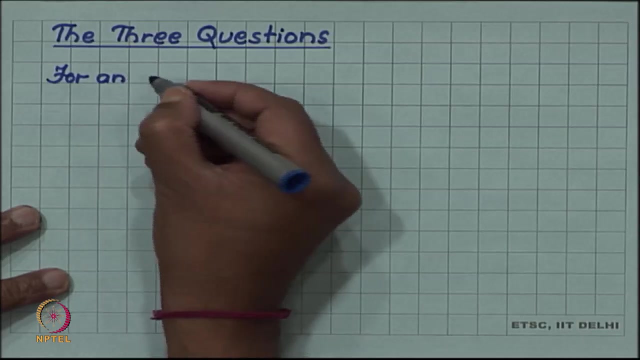 point Now, with respect to any constitution point, three questions can be asked, and let us list those three questions So for any, and the phase diagram can answer those questions. So these questions are important And it is important to learn how to use the phase diagram to answer these questions. So 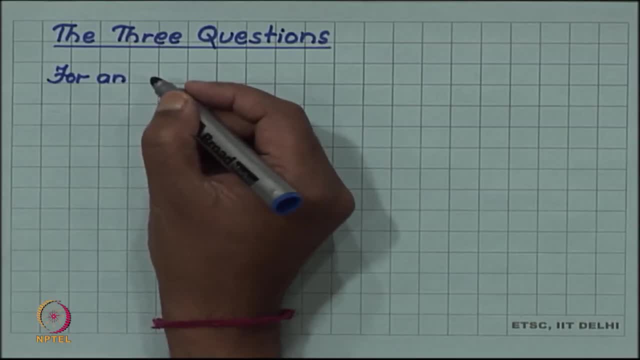 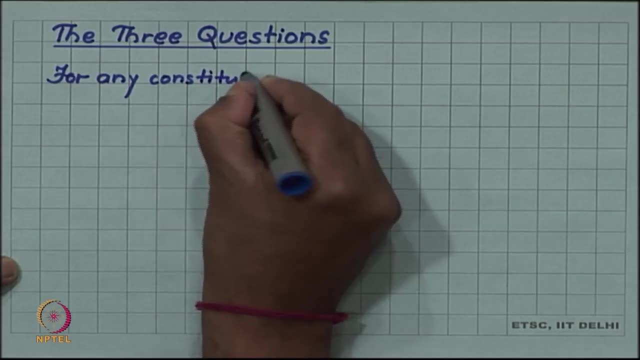 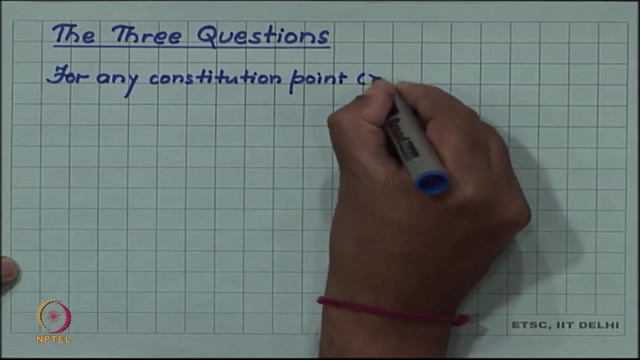 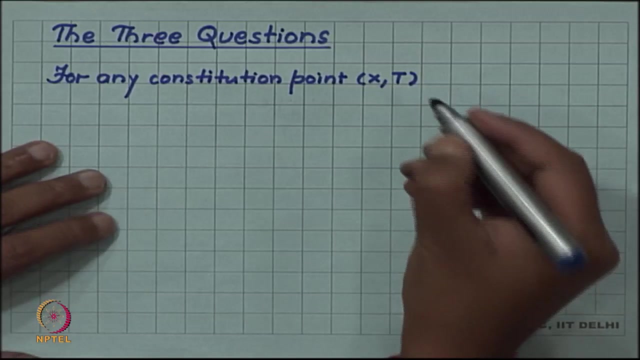 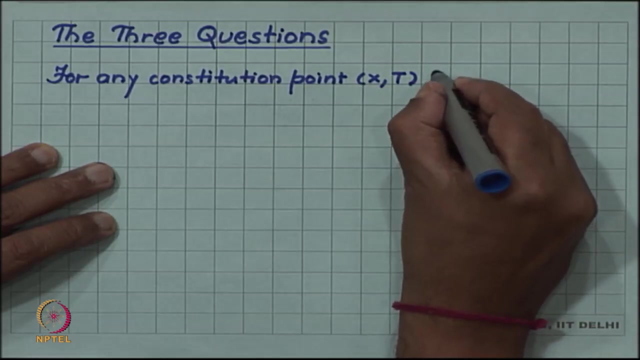 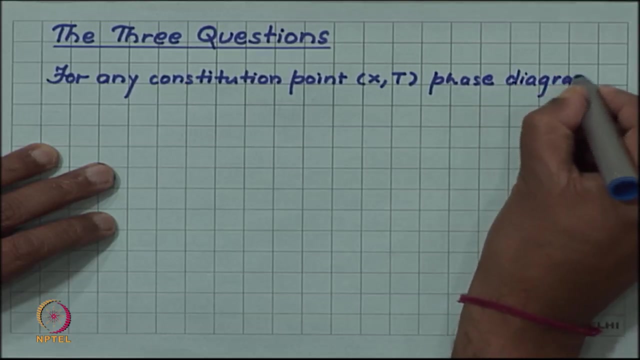 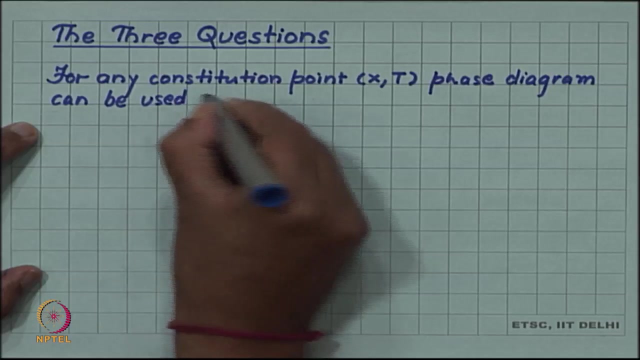 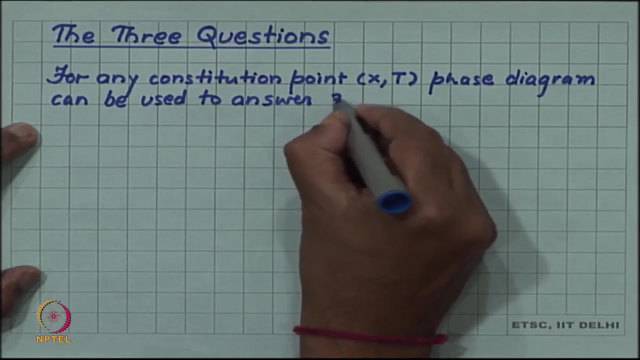 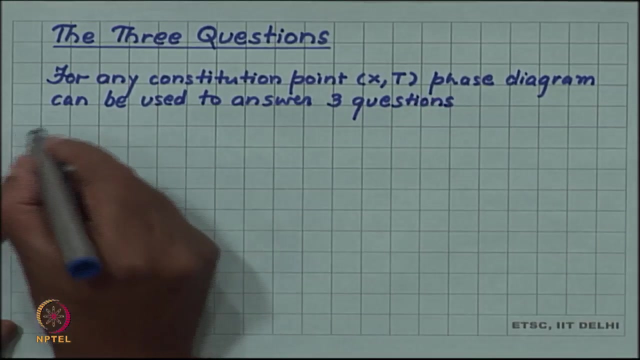 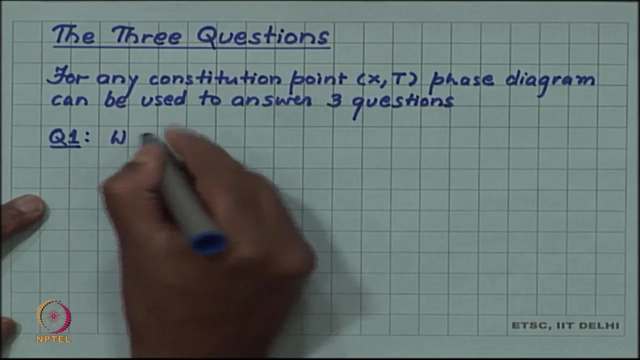 first let us make a list of these questions. So for any, for any constitution, point x, t, we have three questions. So phase diagram can be used to answer three questions. And what are those questions? So let us write that down. Question 1. What are the phases? 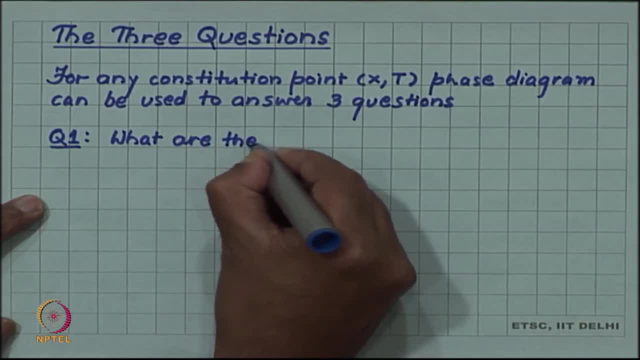 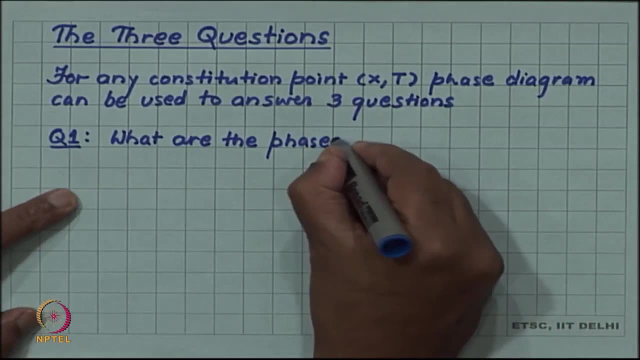 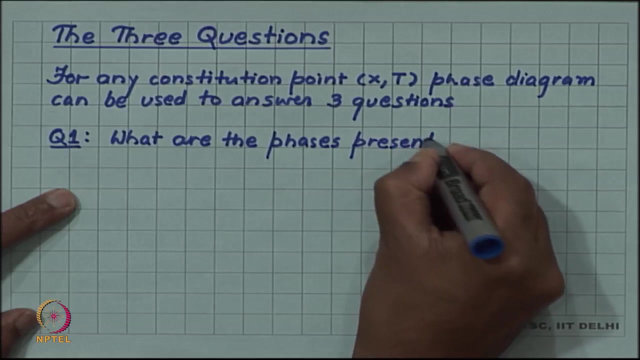 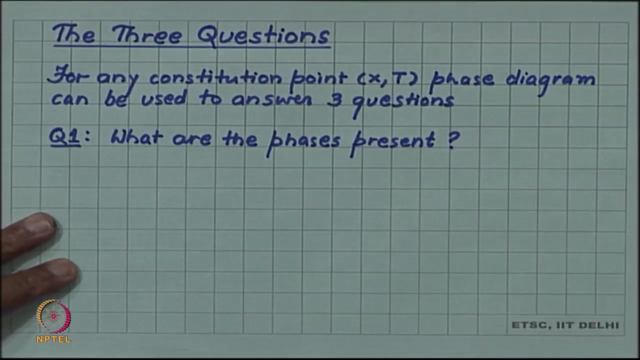 present. So for that alloy, at that temperature, what are the phases present in equilibrium? Okay, So this obviously is the first job of any phase diagram: that with the help of phase diagram we can find what phases are present in equilibrium for any given composition. and 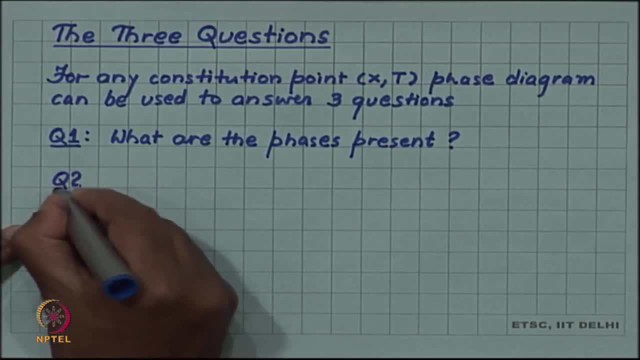 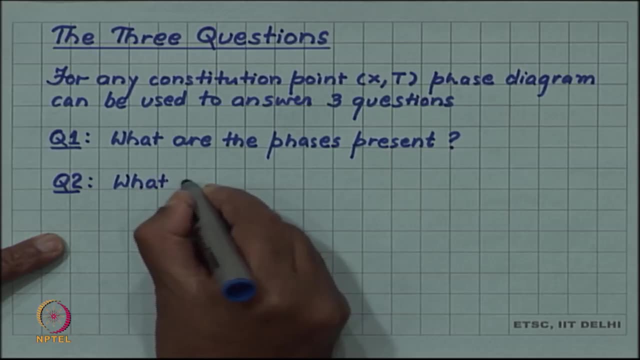 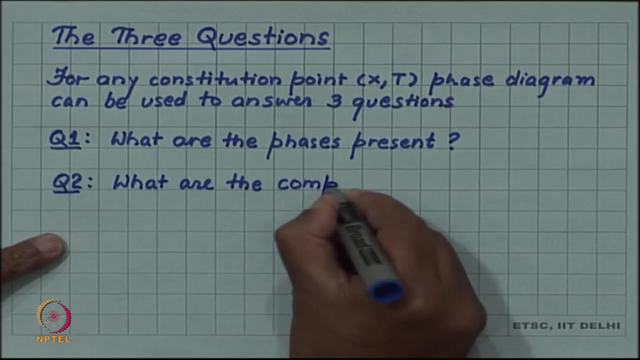 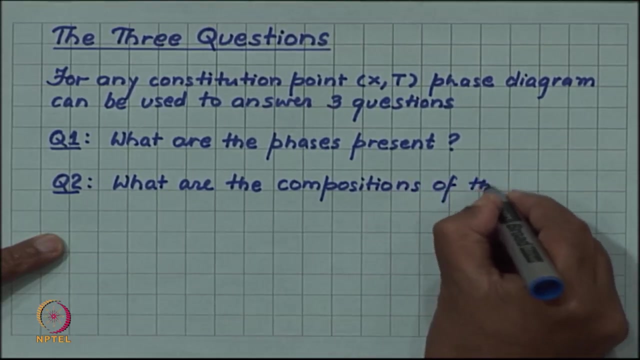 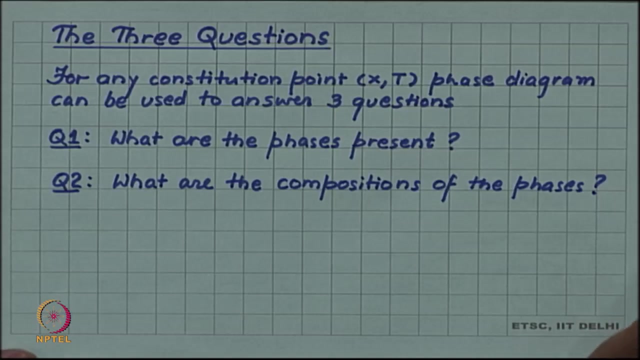 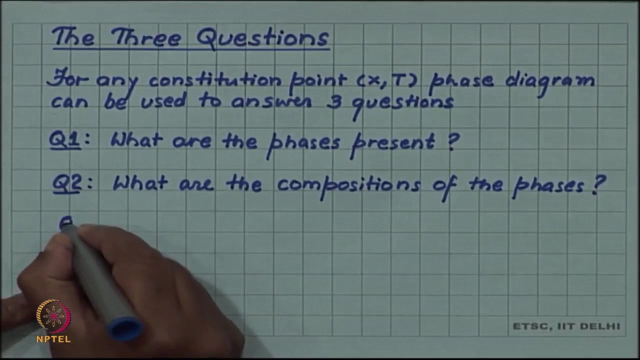 temperature. Another important question is: what are the compositions of the phases present? so once we know what are the phases present- They may be as follows: A single phase or more than one phase- then we would like to know what are the composition of those phases, that is, what is the fraction of components in those phases. and the third: 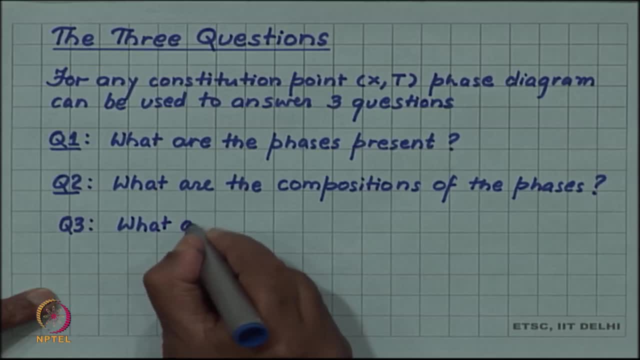 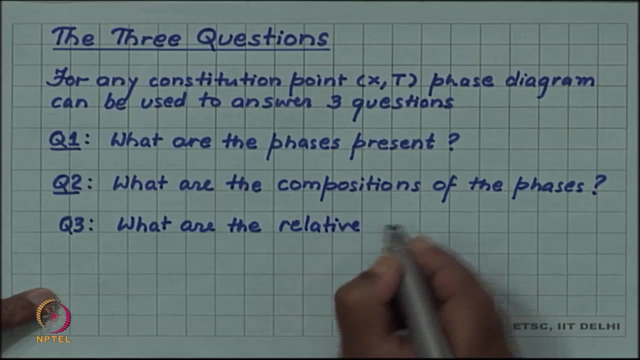 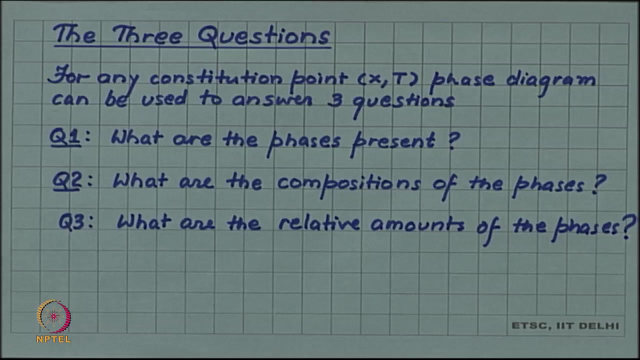 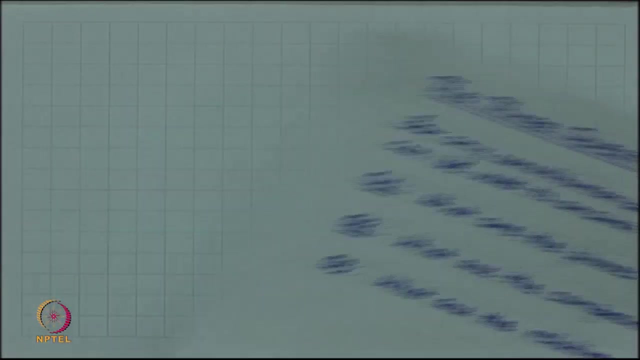 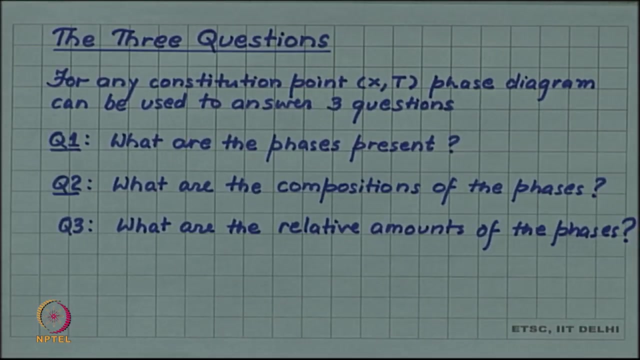 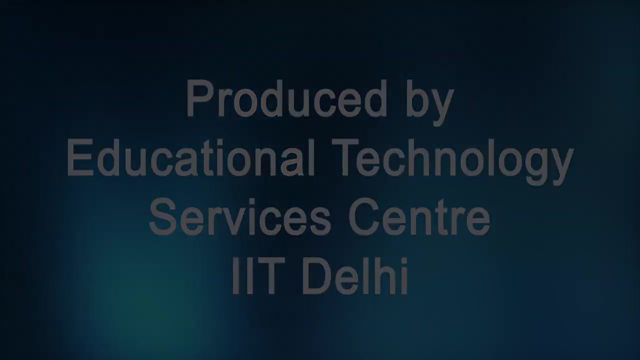 question is: what are the relative amounts? So we will look at the answer to these questions as we go along in the discussion of phase diagram. So we will take these questions one by one. Alright, Thank you very much. Thank you very much. Thanks, Thank you.